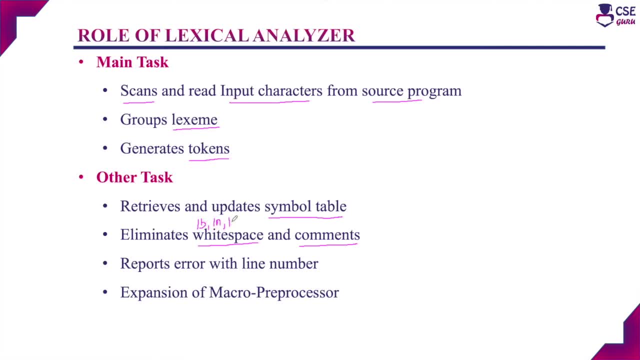 characters: slash n: It is a new line character. slash or carriage return. and slash t- vertical tab. Likewise, if it identifies any white space characters or the command lines, that will be automatically striped out by the lexical analyzer. Since the lexical analyzer will keep track of the new line character, it reports the error message along with the line number. 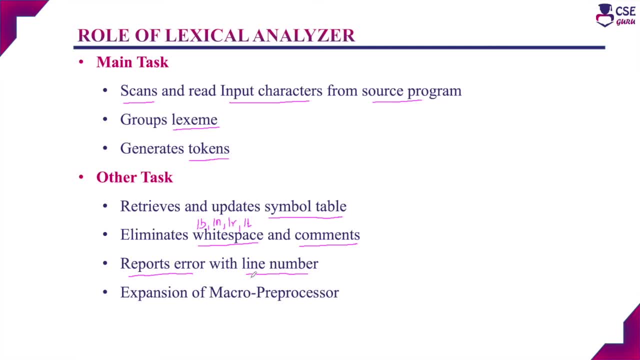 itself In some compilers the lexical analyzer will make a copy of the source program with the error message inserted at the appropriate position, So that will give a proper information to the user to rectify the error easily. If there is any macros present in the source code, that expansion of macro preprocessor is also done by the lexical. 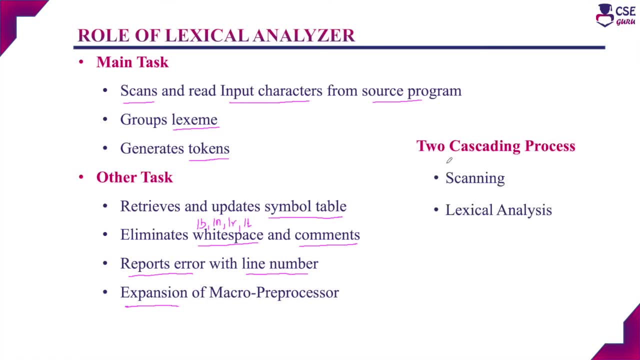 analyzer. So the complete process of the lexical analyzer is a two cascading process. So one is scanning and another one is lexical analysis. Scanning is a very simple process, So it scans only the source code. but the lexical analysis is quite tricky process. It has to recognize 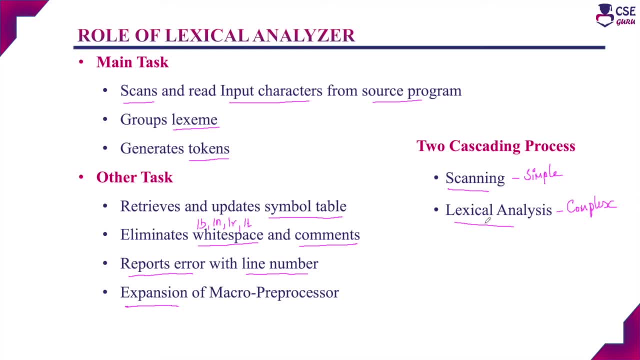 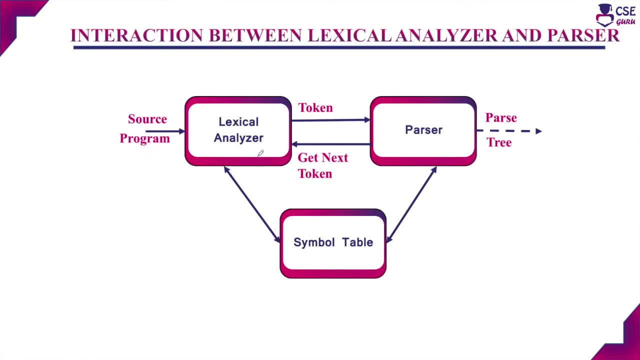 the lexem and these lexems should be converted into tokens. So the maximum processing will be done in the lexical analysis and scanning. it will just scan the source code and it helps to read the input characters from the source code. So it is a very simple process. Next, interaction between 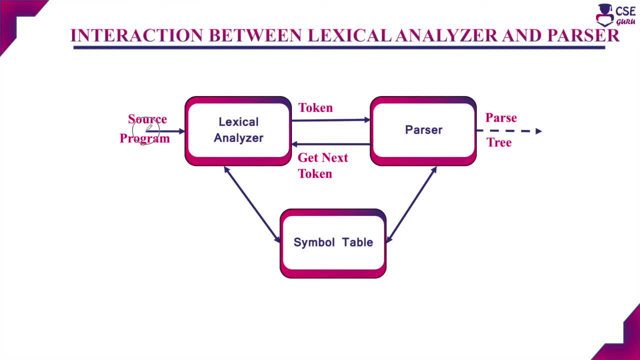 lexical analyzer and parser. The input to the lexical analyzer is the source program. The lexical analyzer will accept the source program and starts to read input characters from the source program. These input characters it will group into lexems and then it will produce tokens comparing these lexems with the pattern. The parser will send a call that is get next. 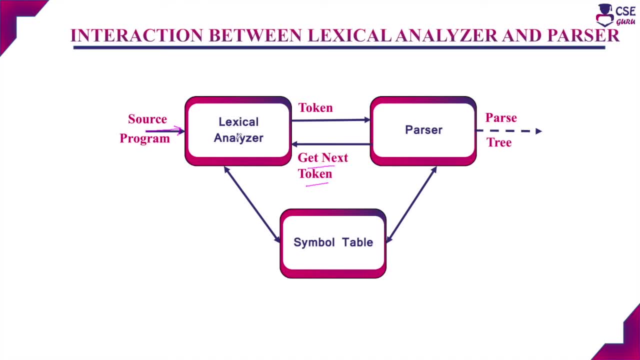 token to the lexical analyzer. Once the lexical analyzer receives the get next token call, it will send its produced token to the parser. Then again the parser will send a call. Again the lexical analyzer will send the token. So this will be a continuous process until it completes the. 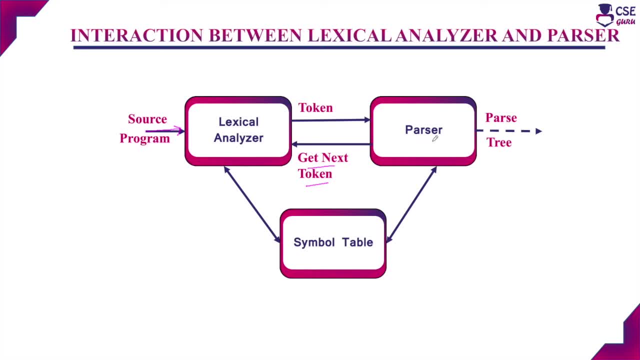 complete source program. Once the parser gets its token stream, it starts to construct the parse tree as the output During the complete process of the lexical analyzer. if it identifies any identifier or subroutines, that information will be updated to the symbol table. This symbol table information. 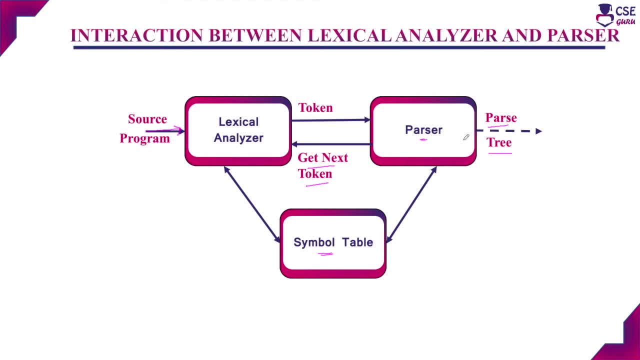 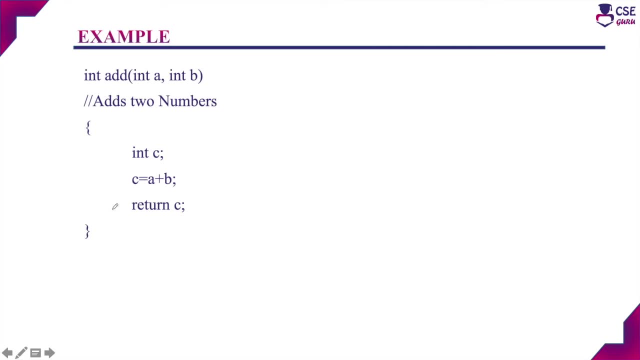 will be used by the parser to construct the parse tree with the help of tokens. So this is the lexical analyzer and the parser. This is the example source code. So in this source code we will identify the lexem and its appropriate tokens. Once the source code is given, the lexical 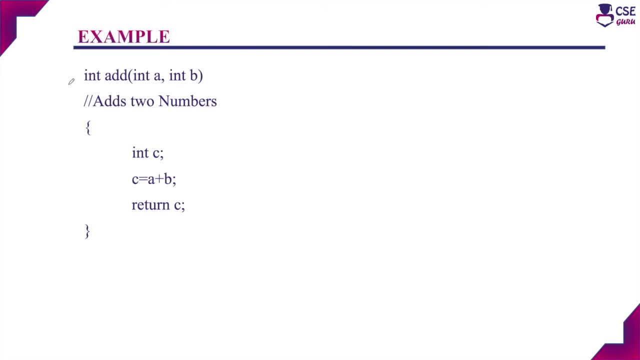 analyzer will start to read the input source code character by character. So first it will start to read int. So this int will be recognized as a lexem and this lexem will be compared with the pattern It will match with the reserved words list. So this lexem, int, will be recognized as a token. 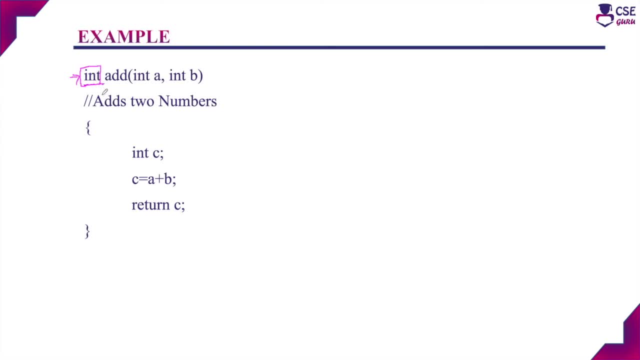 So this lexem int will be recognized as a token name called keyword. Next is a white space character. So the lexical analyzer won't consider the white space character Automatically. it will stripes out the white space characters. Next it will read add. So add is the next lexem and it: 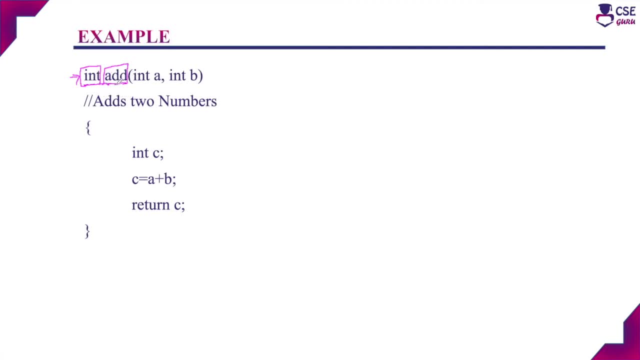 will be compared with the pattern. It matches with the token name: identifier. Next, open bracket with the token name. punctuation symbol: Int is a keyword. A is the identifier, Comma is the separator or under punctuation symbol: Int is a keyword, B is the identifier and close bracket. 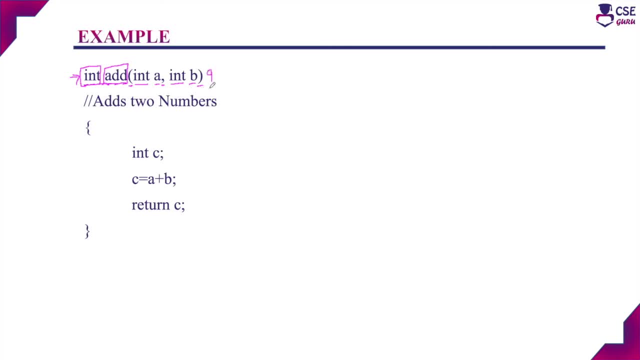 is a punctuation symbol. So if you are considering this first line totally, there are nine tokens. Next, after completing this first line, you will move to the second line. So the second line is a comment line. so the lexicon analyzer automatically stripes out the whitespace characters and. 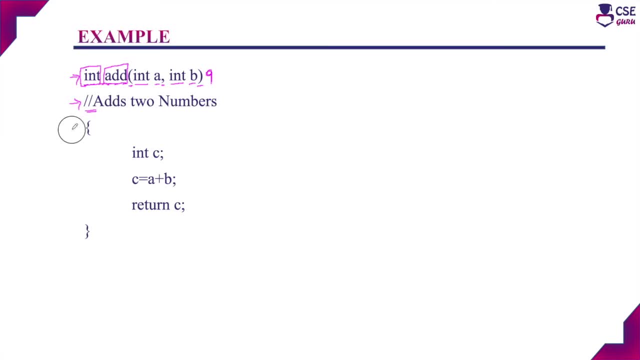 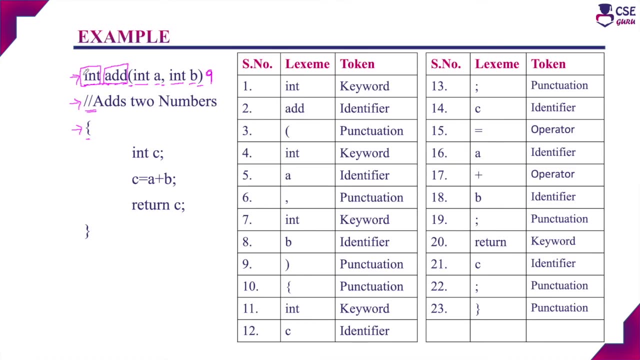 comment lines, so it won't consider the command line. next it will move to the third line and it will read the operation code. This is the first argument. Next it will take text. it will move to open brace. This open brace will be recognized as a token punctuation symbol. So likewise if 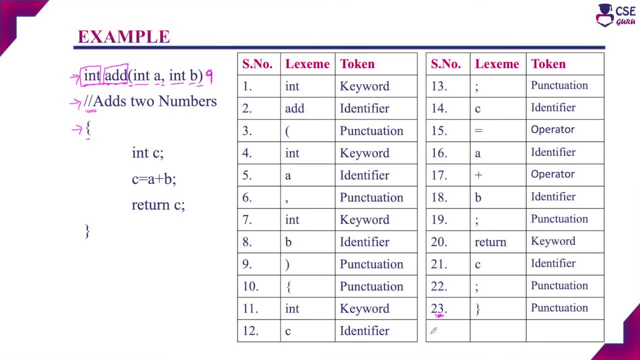 you are considering totally. there are 23 tokens present in this example. The lexical analyzer will read the input characters present in the source code and group them as lexems. So for each lexem it will compare with the pattern to describe the appropriate token. Okay, next issues. 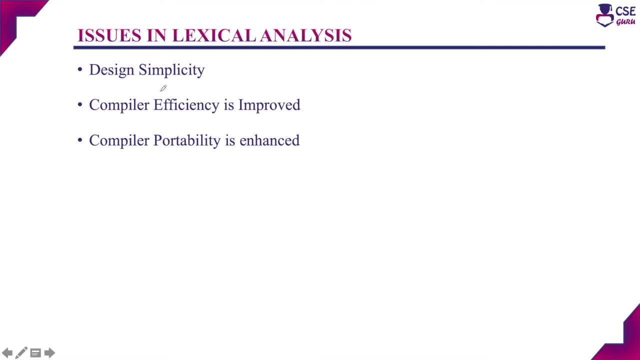 in the lexical analyzer. There is a main question why this lexical analyzer and the parser is separate. So the first reason is design simplicity. because the lexical analyzer has to do more tasks. It has to read the input characters, identifies the lexems and convert each lexem into appropriate.